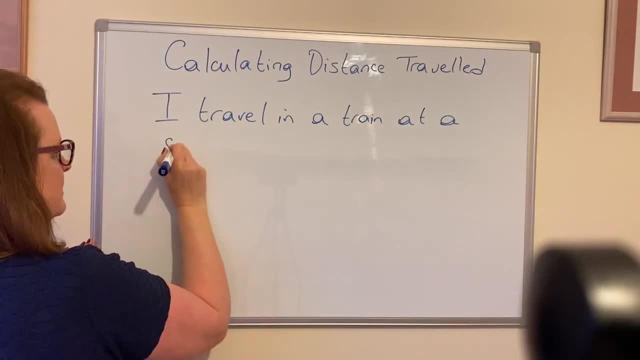 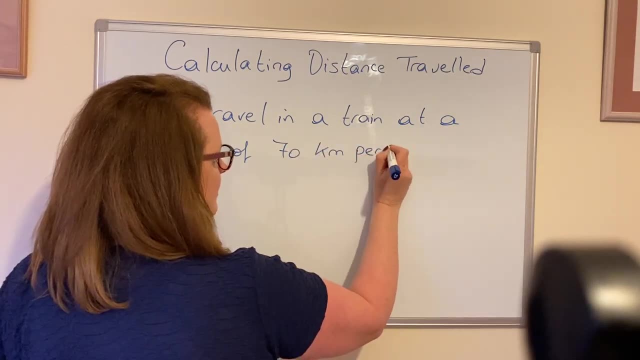 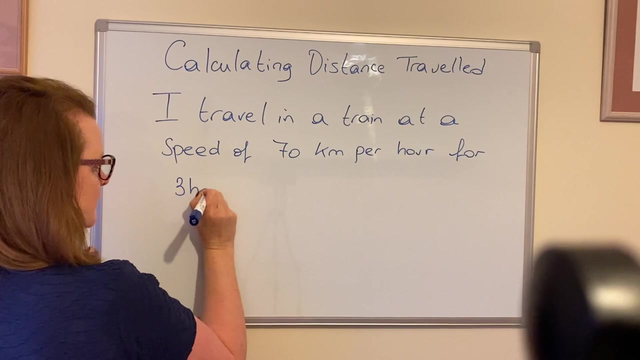 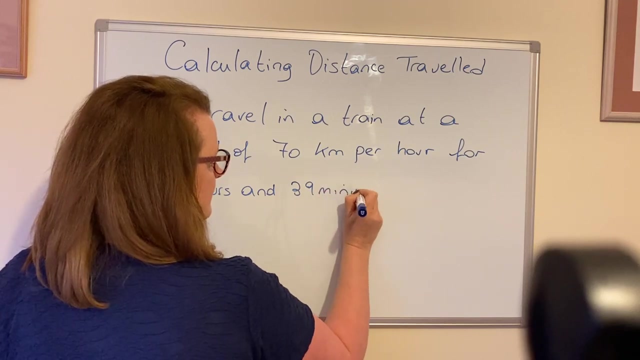 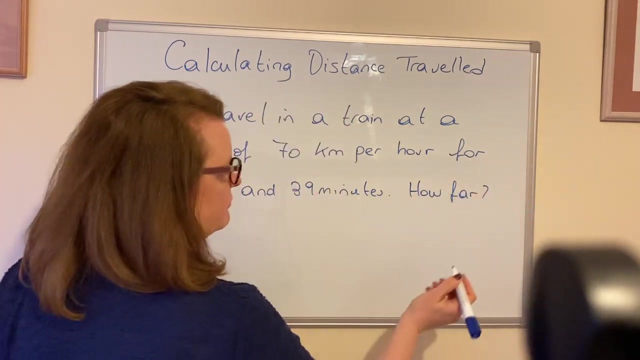 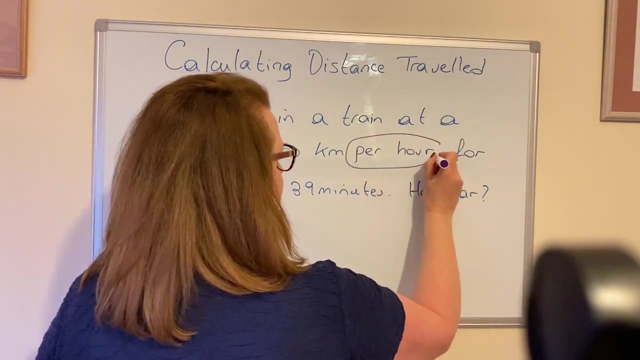 And the train's going at a speed of 70 kilometres per hour for 3 hours and 39 minutes. Same question: How far do I go This time? the units of time are not quite matching. There I have an hour, But here I have hours and minutes. 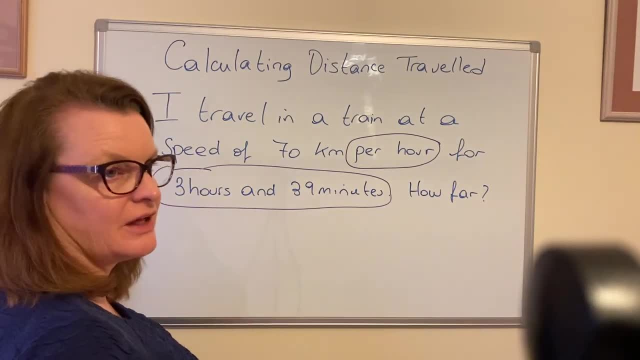 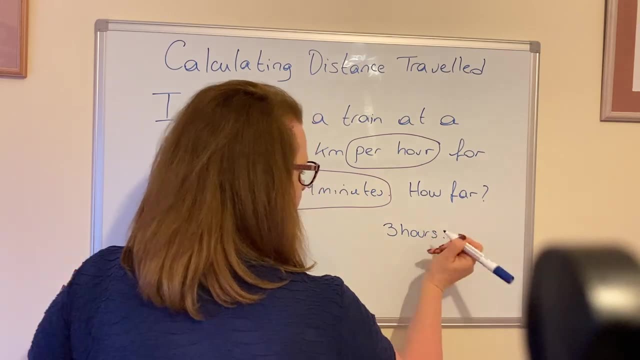 So I'm good to go, I'm not good to go. I need to convert that into time as a decimal, as we did for the first lesson. So for the first lesson we kept the three whole hours over to the side and we took the. 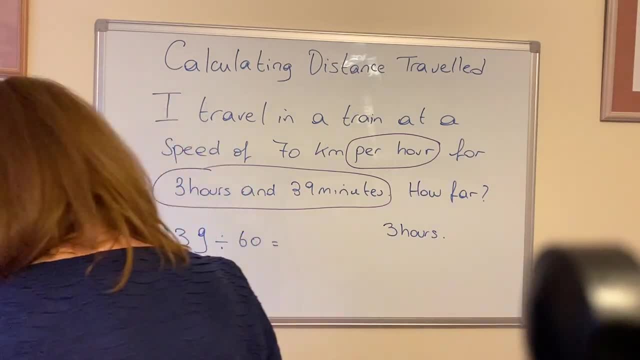 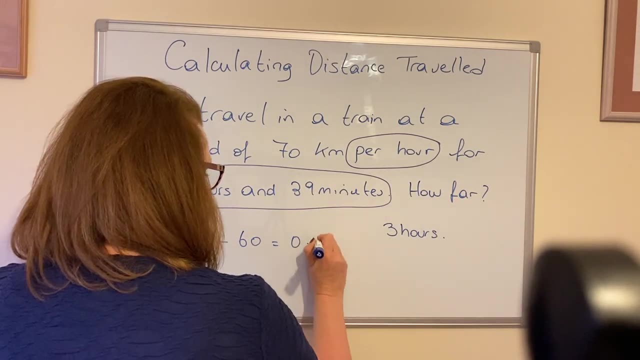 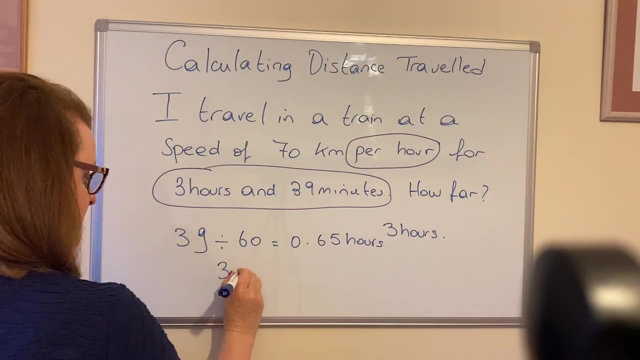 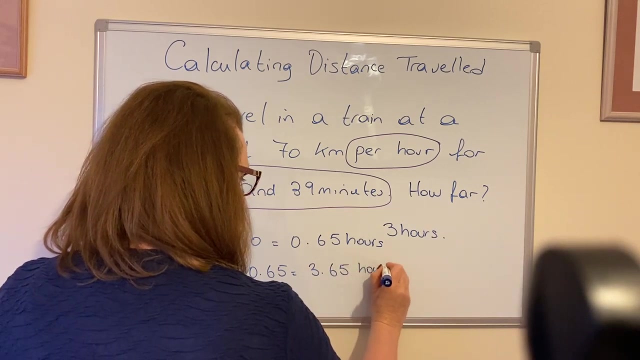 39 minutes and we divided it by 60. to put it into a decimal: 39 divided by 60 is 0.65. Hours. So if I add that to my three I get 3.65 hours. Now I've got hours and hours that matches. 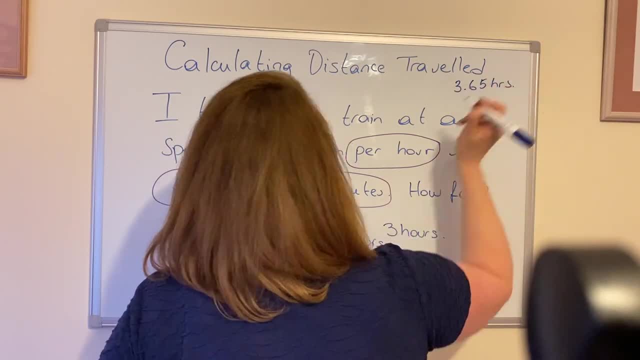 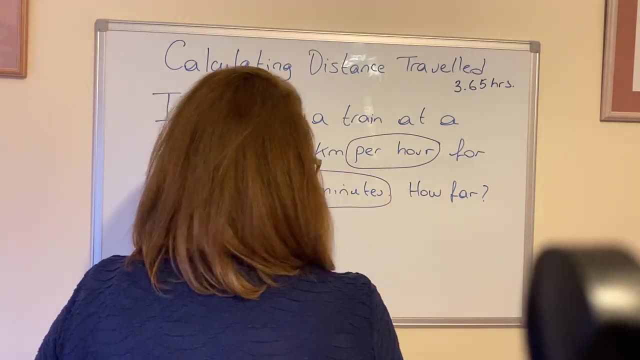 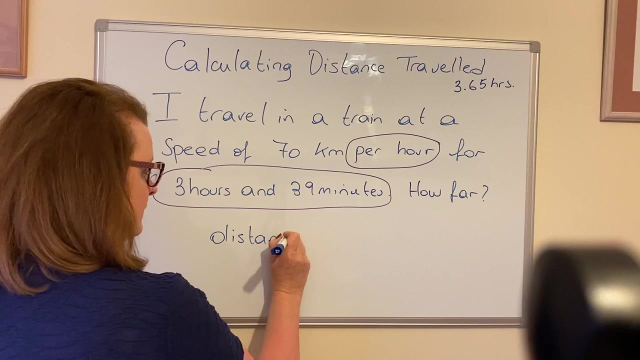 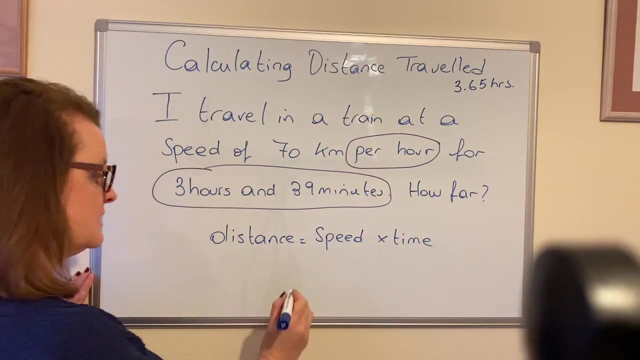 And I'm going to write my 3.65 hours up here so that I can rub it off the bottom and create myself some space to finish. So now we need to go back to our formula. Distance equals speed, times time. My speed from the question is 70.. 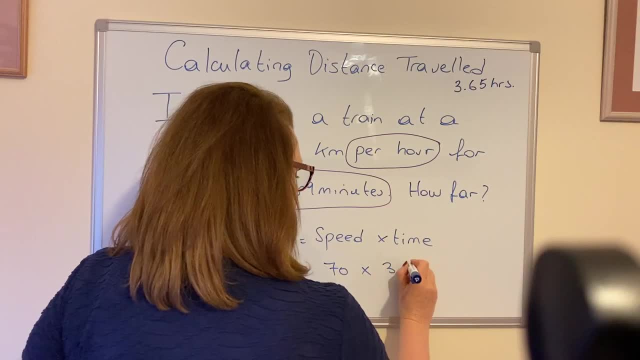 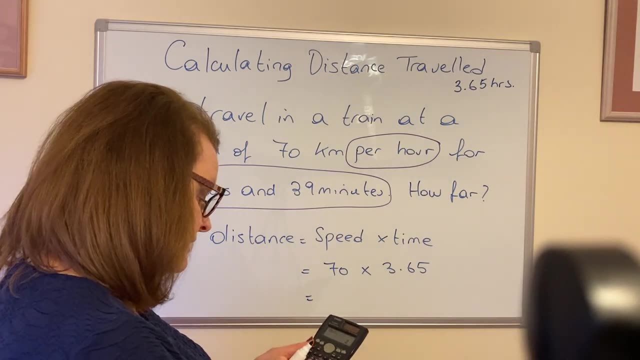 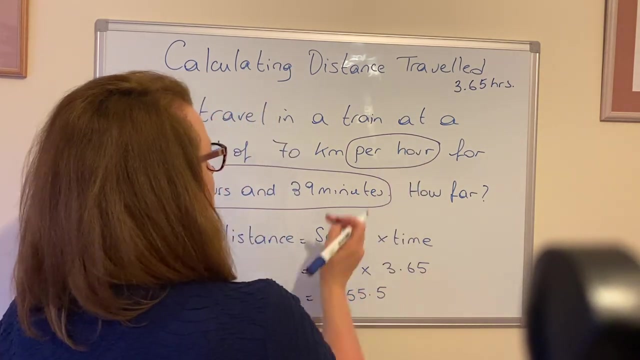 I need to multiply it by 3.65 hours. Again, we're allowed to use a calculator to do this And I get 250. And 55.5.. Look to the speed. The distance, part of the speed, is in kilometres.